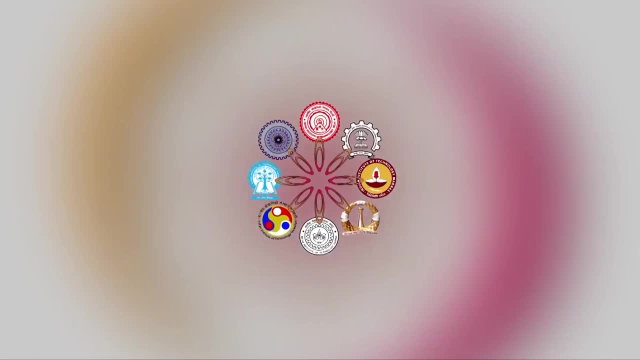 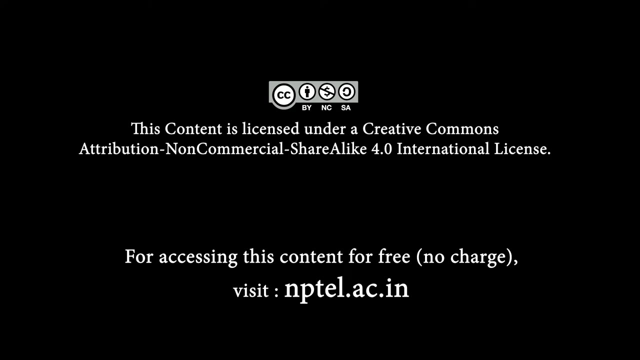 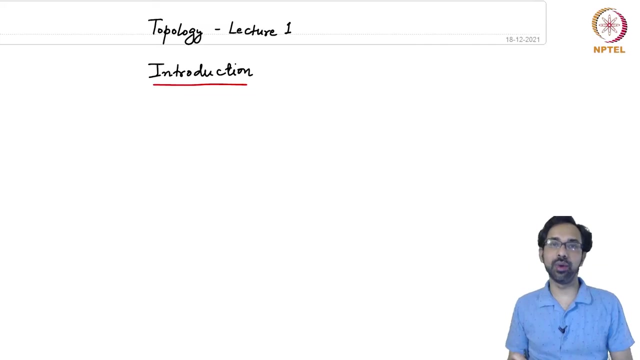 Hello and welcome to the first lecture in topology. Today we will answer the question: what is topology, What is topology? But before we answer this, first we should know what kind of topology we are talking about. So there are various topics related to topology. 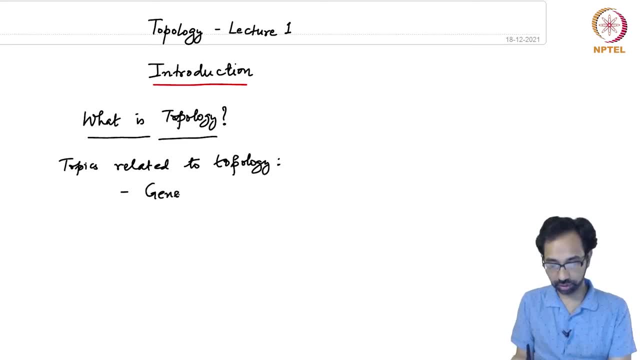 So first one is what's called general topology or point set topology. Then there is also algebraic topology, And then there are others, such as combinatorial topology, Ah, differential topology, et cetera. But in this course we will only be concerned with the first one, which is general. 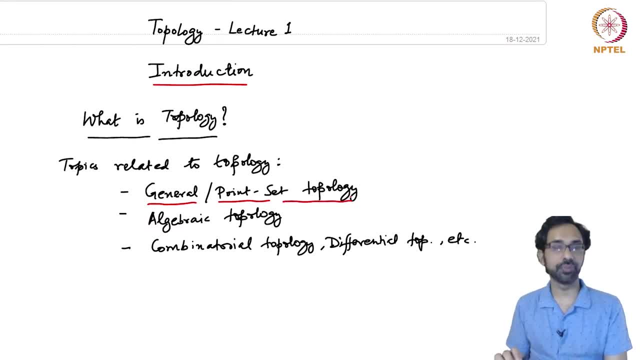 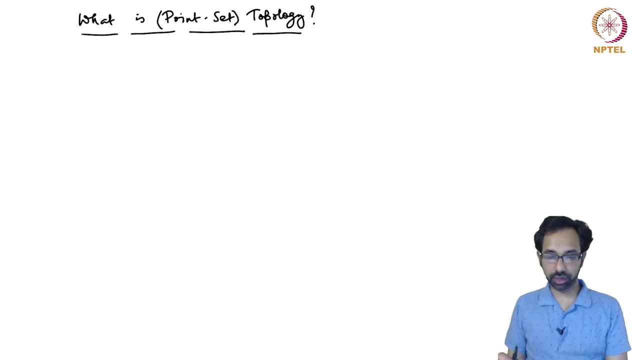 point set topology. So in this course is about points of topology. So what is points of topology? Ok, so let's answer the question: what is Points of Topology? and ah, I wanna only use this one term, topology, to refer to points of topology. So let's list the main features of this subject. 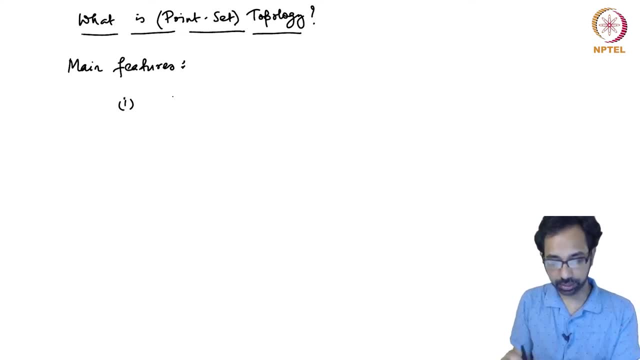 So the first one is that it is a gateway to geometry. and what do I mean by a gateway to geometry? It means that topology studies geometrical objects, studies geometrical objects, but it is something more, in some sense more fundamental or more basic. It is more fundamental. 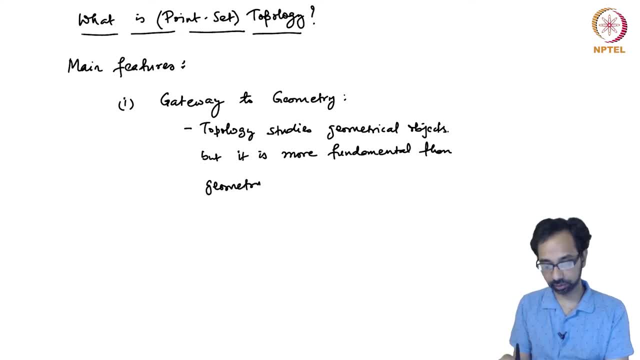 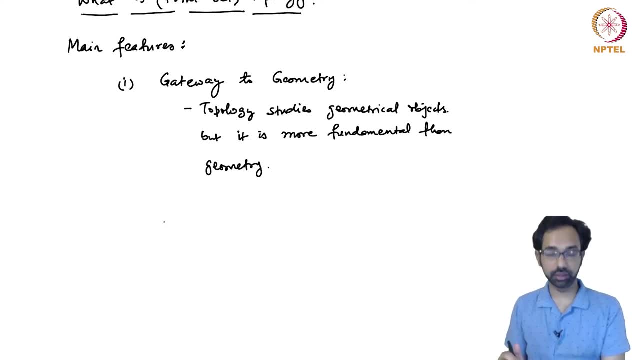 than geometry. So historically, topology started as a study of usual geometrical objects that we know, like polygons etc. But eventually it became an abstract subject on its own. So it is used as an abstract project to sleeping Pokey, multipse, Milky Way. That that's another great. 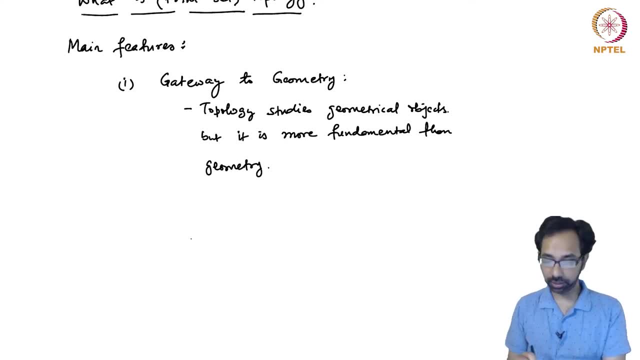 to study the usual geometrical objects that we are familiar with. but it is also something that lies, that becomes a platform for studying geometrical objects. but it is also different from geometry. how is it different from geometry? so we can go to a new page. so in geometry we 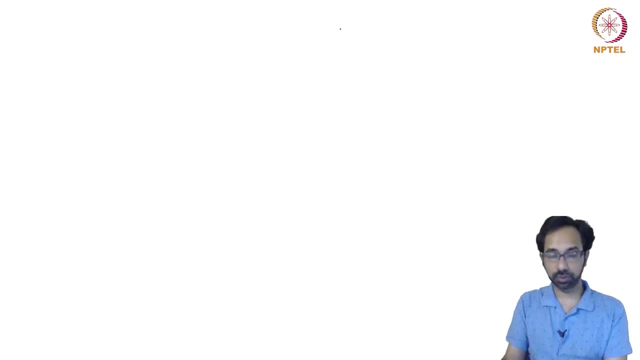 study curved objects. so, for example, this is a curved object, okay, and in geometry these two things are considered different. and this is a flat object. and in geometry these two things are different. different why? because the first one has a bent shape, it is curved, and the second one- the one below is- is flat. it has no, no bending right. so in geometry these are: 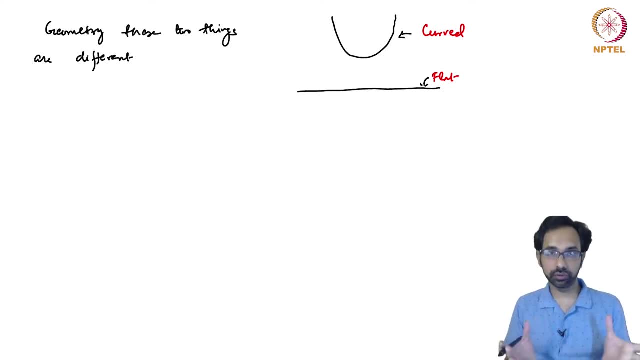 different and geometry studies the amount of this bending or curvature. it's called curvature and it distinguishes things that have different curvatures in you have, you might have already seen euclidean geometry, where you have studied things inside a plane like triangles or polygons, and you might also have also 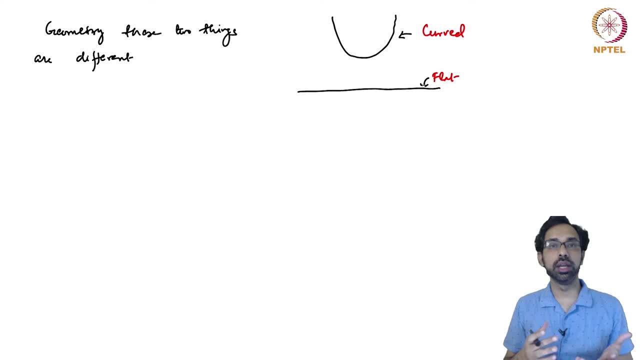 have seen coordinate geometry, where you study mathematical objects, geometric objects that can be expressed as equations, and all of them have a precise shape. that the triangle has a precise shape, a polygon has a precise shape, and if you bend it in some way then that shape changes and the geometric object is is different. but in topology all these things are equivalent, are the same. in topology they are the same. and what do i mean by same will be explained later. 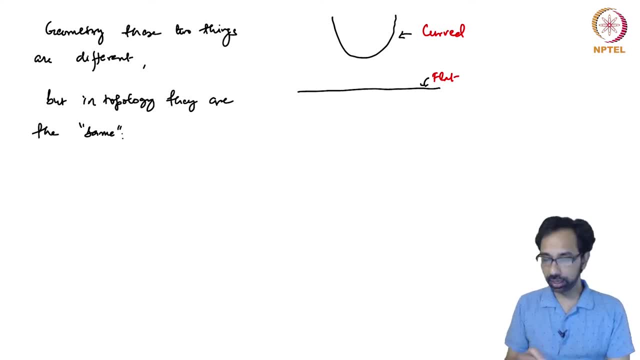 we will make it very precise. what do i mean by this? and and these two things, the curved one and the flat one, are the same in topology. so it is topology is a gateway, something more fundamental to geometry, and it is also different from geometry. okay, the third one, the third main feature of 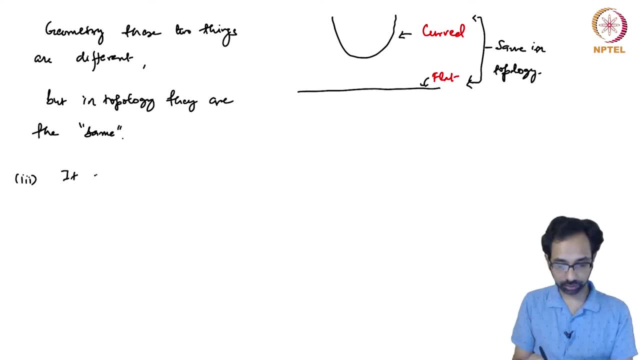 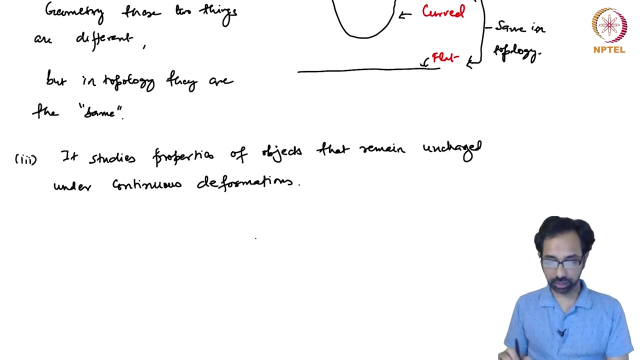 topology is that it studies properties of objects that remain unchanged under continuous deformations. continuous deformations, and what do I mean by this? so an example of this feature is: is the circle and the square, so both this, these things, have this kind of hole in them. okay, so I'll call this a. 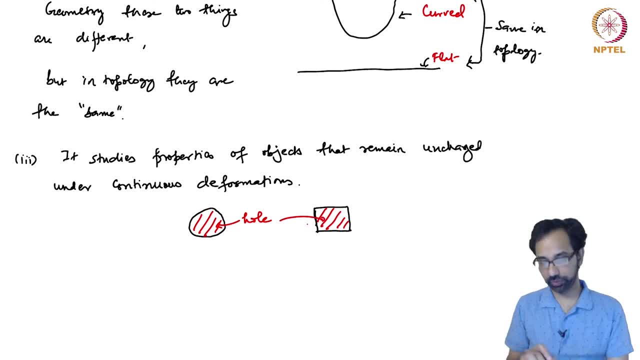 hole. and we see that if you, even if you stretch your circle in some way, so you can deform your circle in whichever way you like. you can make it a square, or you can make it another square, or you can make it another square, or you can make it another. 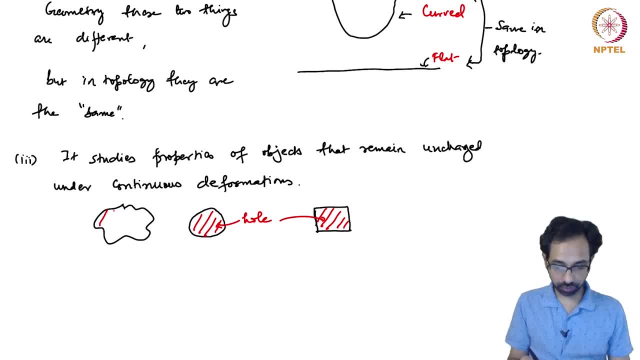 shape, but this number of hole that we have is still the same. right, it's still one. so all of these have they have one, and this is an example of something that remains invariant under continuous deformation. so you can think of getting this, this shape, from the circle by deforming various parts of the circle, and you can also 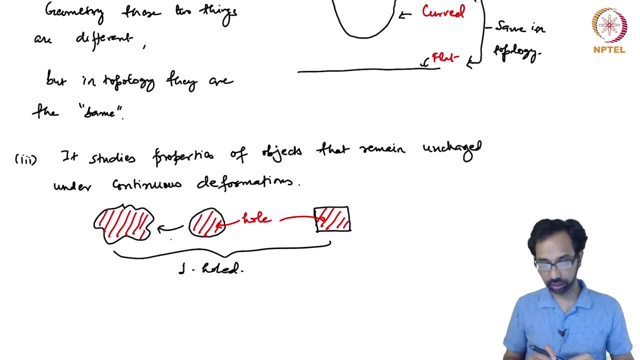 think of the square as being deformed from a circle using continuous deformation. and what do I mean by continuous? it just means that you are not allowed to have any discontinuity in this, in this deformation process or, in informal language, you are not allowed to tear it apart. so, for example, you cannot. 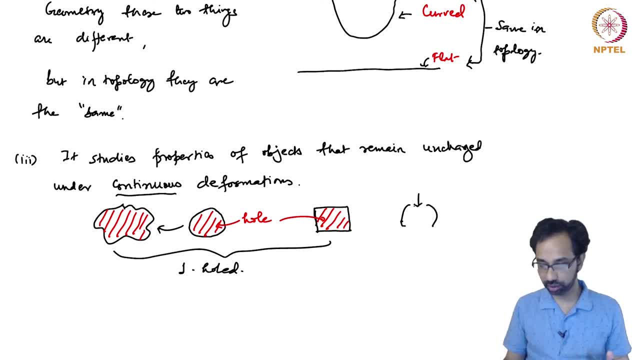 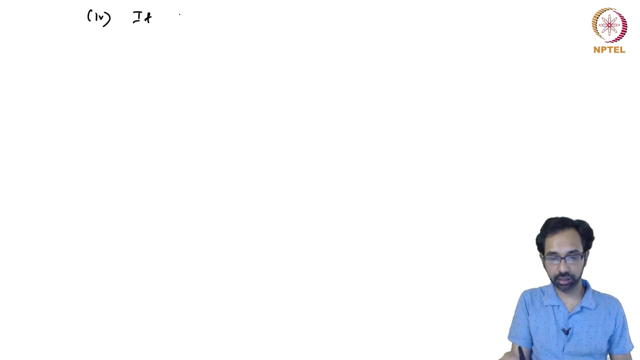 do this from a circle, so you cannot have a tearing of the circle. it's not allowed. so this is what is meant by continuous deformations. so under continuous deformation, some properties of topological objects remain unchanged and topology is used to study these properties. okay, another main feature of topology is that it 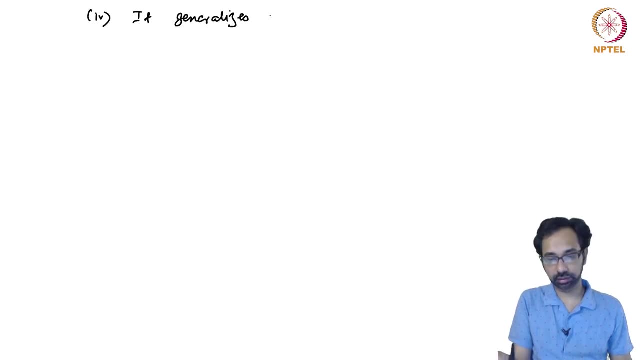 generalizes and unifies ideas such as continuity and convergence. by convergence I mean limits. so if you have studied calculus, you have seen both these concepts of continuous functions and and limits of functions. and topology generalizes and unifies these, these ideas, to an abstract setting. so what do I mean by generalizes? so usually in calculus? in calculus, 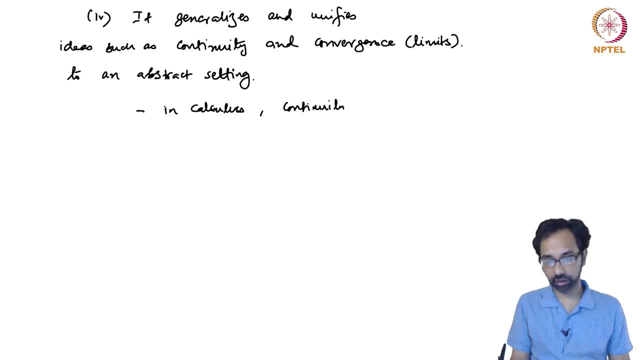 We have seen, continuity and limits are studied for real numbers, and what topology does is? it allows us to talk about continuity and limits in a wide variety of other settings that are different from real numbers. So in that sense, it generalizes these ideas. What does it mean by unifies? 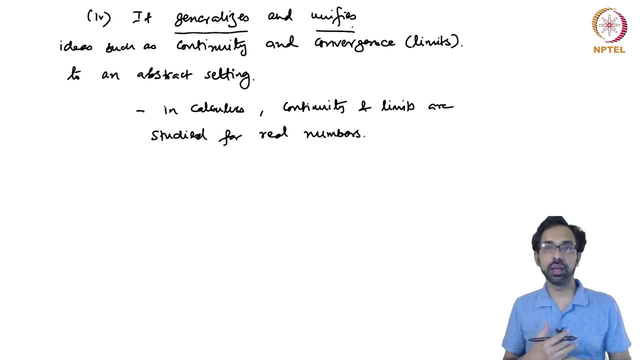 It means that the same definition, the same way to express continuity and limits, can be used for various different things. So not only does it generalize to other, more different settings, It also allows you to talk in the same breath the ideas of continuity and limits, meaning that 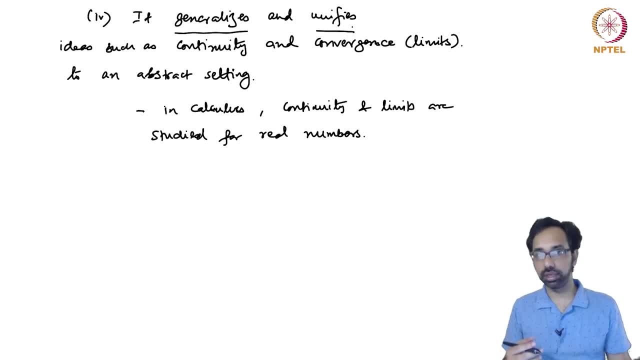 the same definition for continuity and limits works for, let's say, any other space, and the same definition works for real numbers as well. So in this sense, it generalizes and unifies these ideas. Lastly, it gives. What does it mean? 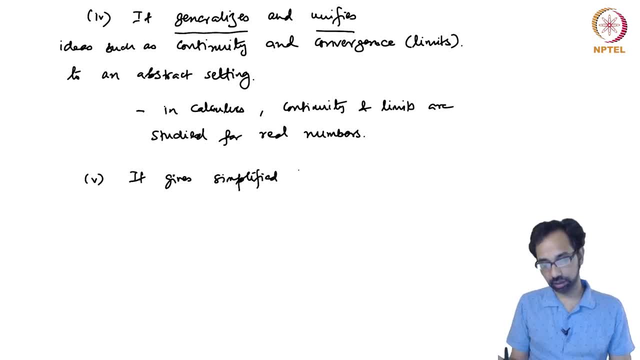 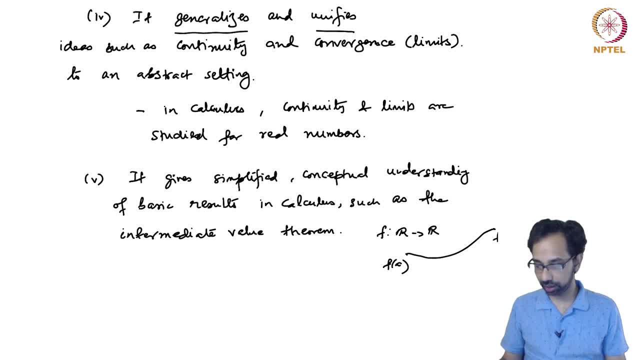 values between f and f, then there exists a point c which So, given any point in between these two values f a and f b, So these are the two values f a and f b, given any point in between there exists a c, such 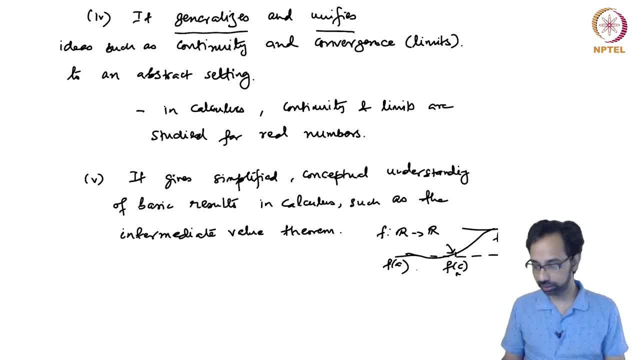 that this point can be expressed as the range of f, So it is of the form f of c. So this kind of theorems are very basic to calculus and topology. Yeah, Yeah, By conceptually understanding, meaning that it allows us why these things are true. 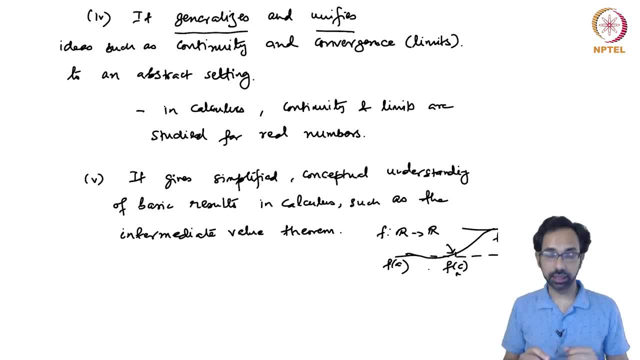 And in that sense it gives you a simplification of these concepts. So, uh, Then we can also talk about 14. Then we know why these things are true. Then we can also talk about these things in a more abstract, more general settings.